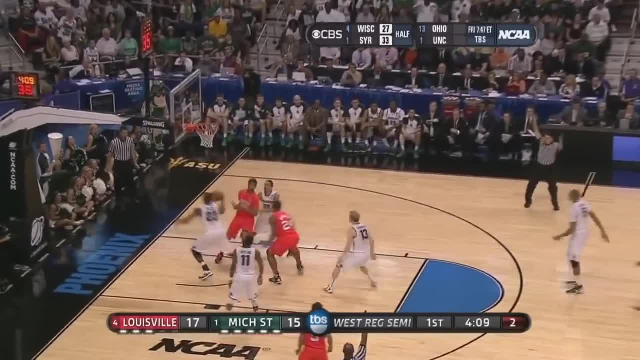 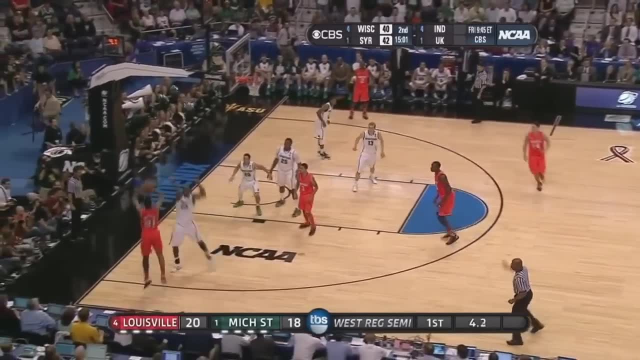 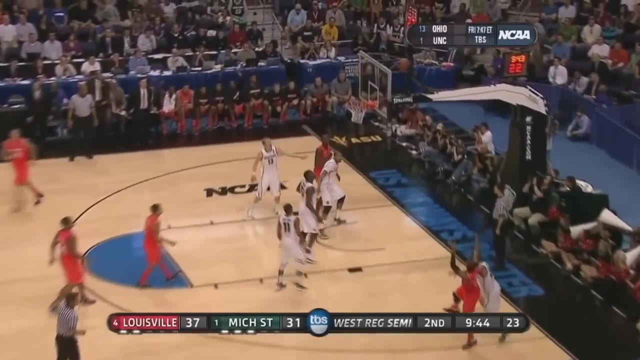 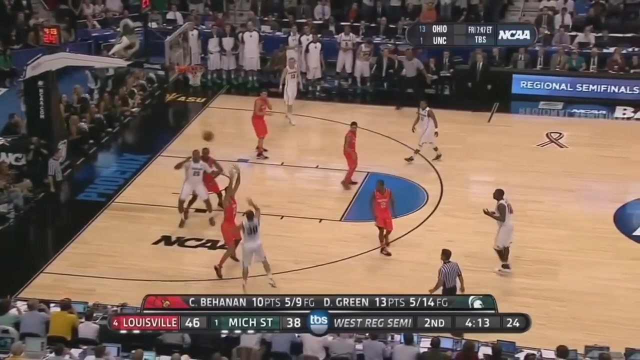 Seba James Finds some breathing space and knocks down a triple To the 25-footer. Here they go. now Swapshire with a three. Good, This is Chris Smith with a three Wood. Swapshire comes in and defends. 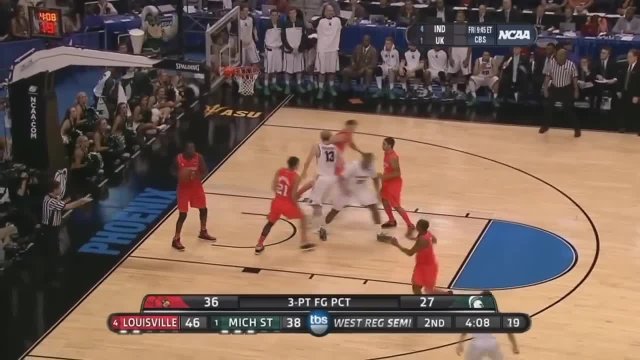 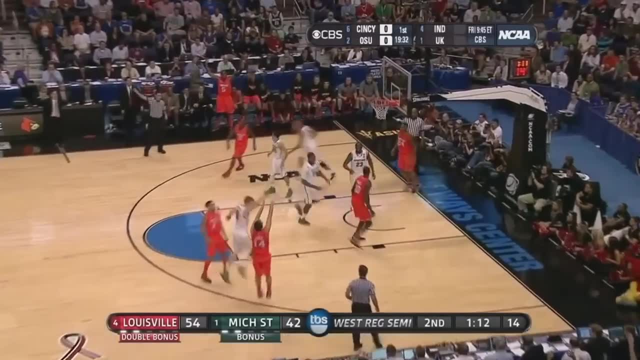 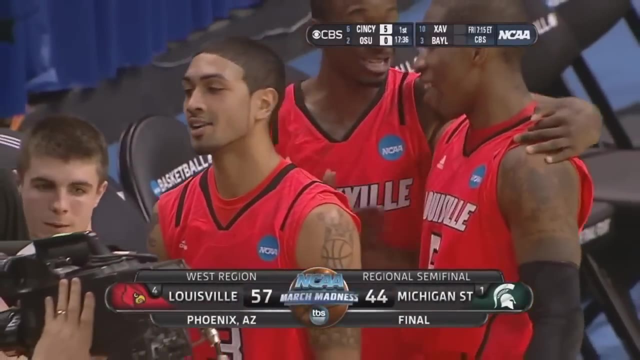 And Nick now goes up against James. Another block, He's got six. He is indeed playing handball. You've got to stay on guard. Seba Carrot, for three. I can't be saved. My, my, my, my. 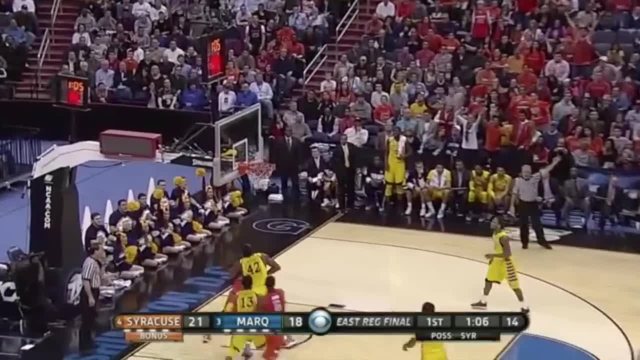 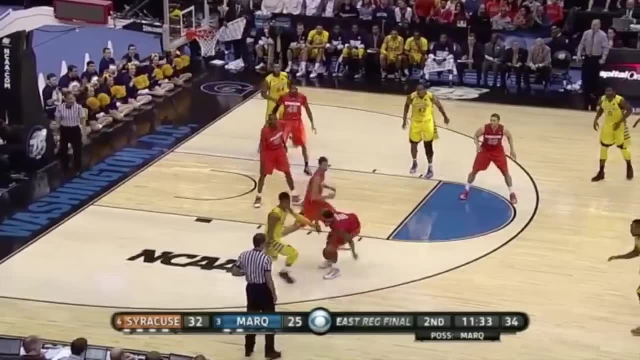 Late in the half, Michael Carter-Williams looking and finding James Sutherland for three Syracuse up by a half dozen at the half 24-18.. Later It's that man, again Michael Carter-Williams, after the great CJ Farris. 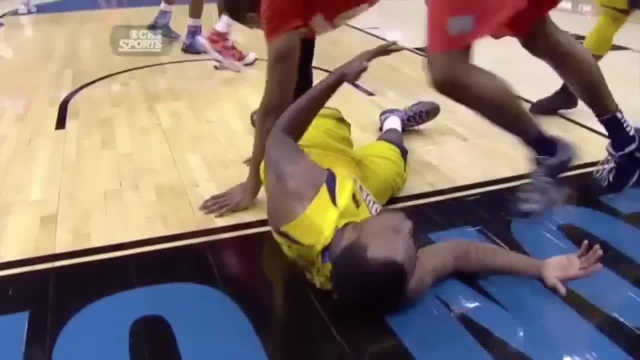 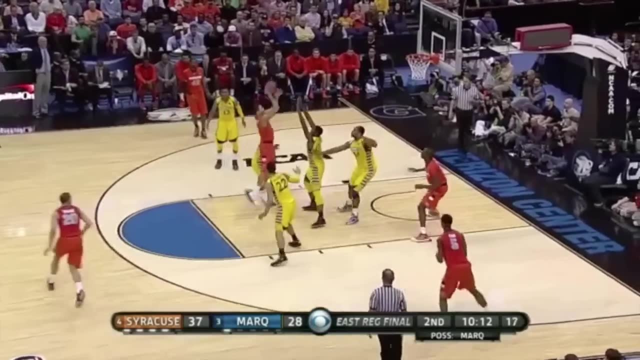 Getting it over to James Sutherland, going strong to the rack, laying it in and drawing the foul. Guess who gets landed again on top of It's? Cadogan, one more time. Orange up by 10, Michael Carter-Williams: just a superstar in the making. 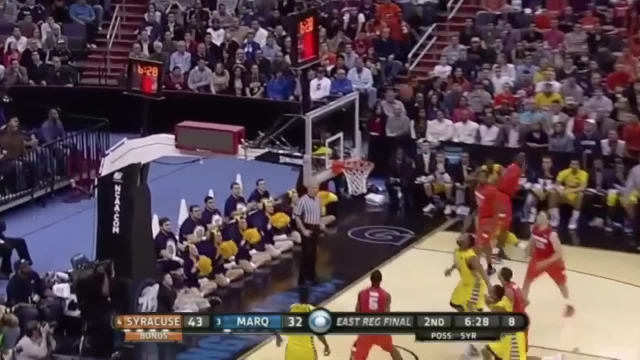 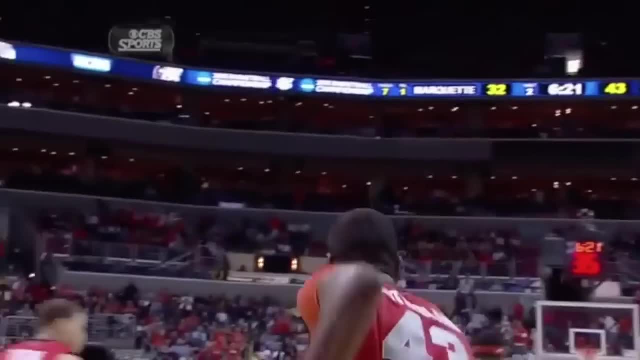 Tough floater: 12 points, 10 rebounds, 5 assists on the game. Cuse up by 11, later Marquette missing the 3.. We go the other way and race into the bucket and throwing it down is Sutherland. 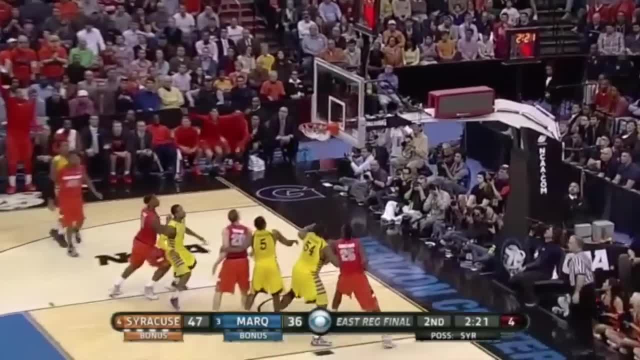 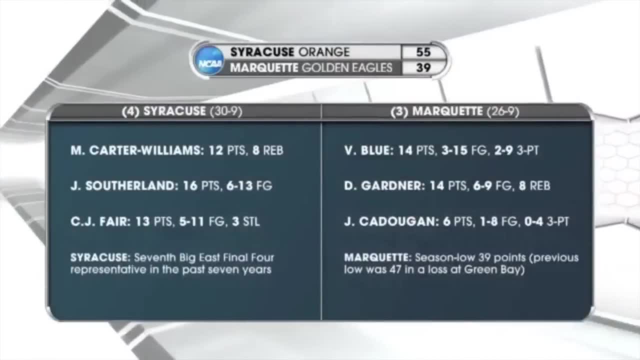 Sutherland led the way with 16 points on the game. he can do it from outside as well: Defenders draped all over him. he drills the shot and Derek Coleman's pleased Syracuse wins this one by 16 points. Marquette shoots 23%. as a team, it's the Orange's fifth. 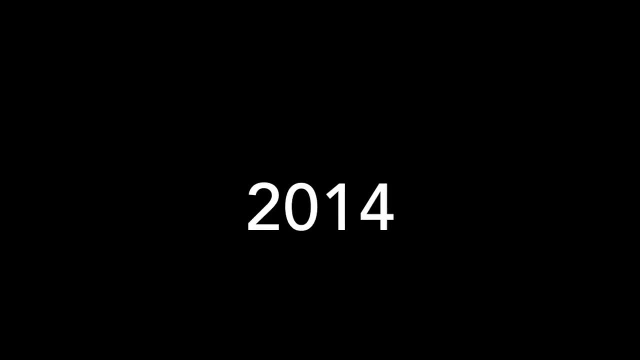 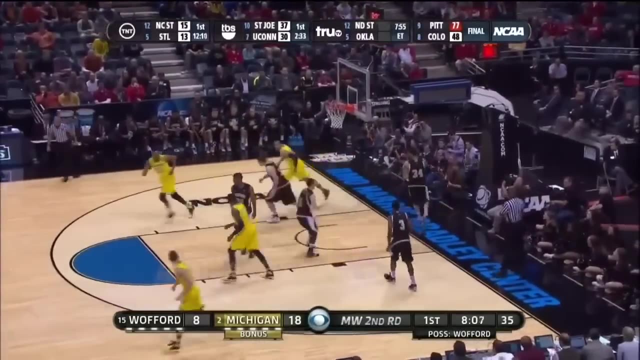 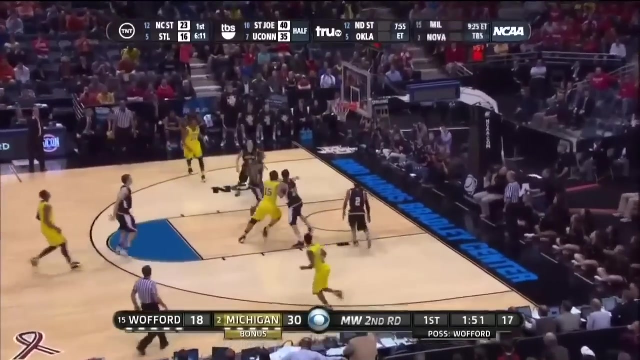 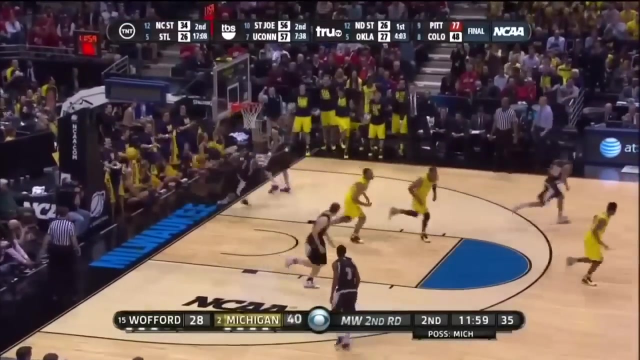 Final Four. they win it 55-39.. It's to play this first half, Robinson over Newman Booker. nice ball handling huh Walton. baseline: the slam by Horford. we have not seen many backdoor cuts on the baseline. 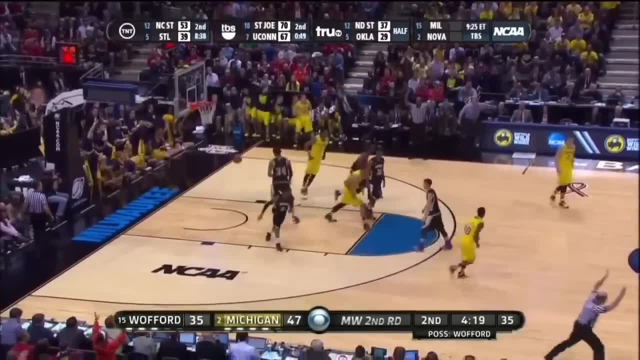 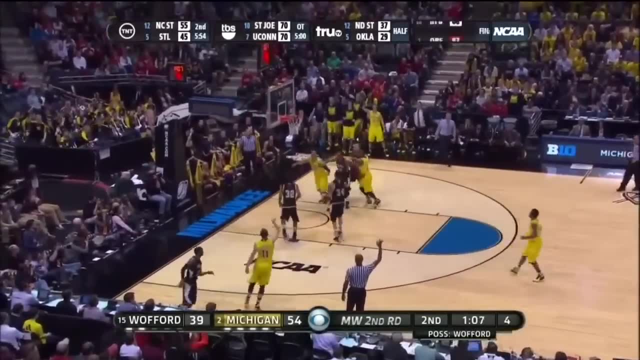 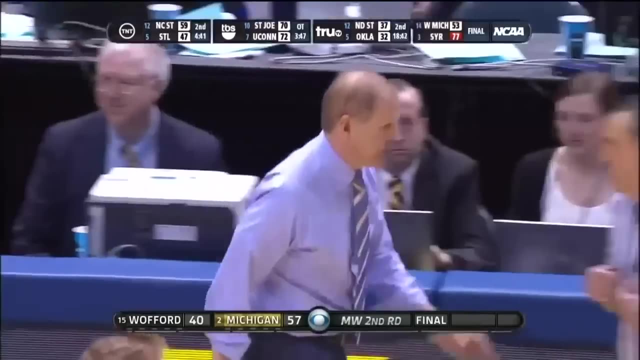 at all for the B-line squad, the third on a three. Walton gives it up. Skoschkis open one for shooting practice: a three. how about one for the? A year after going to the NCAA championship game? Michigan begins its run in the 2014. 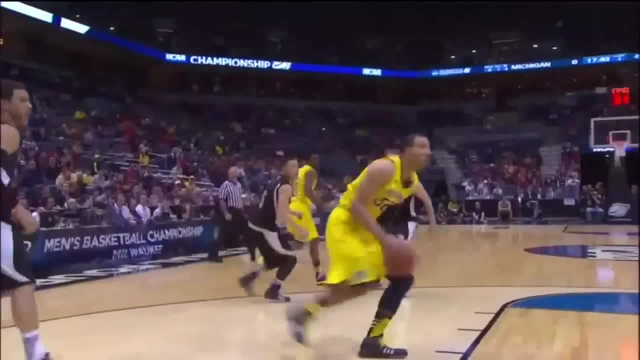 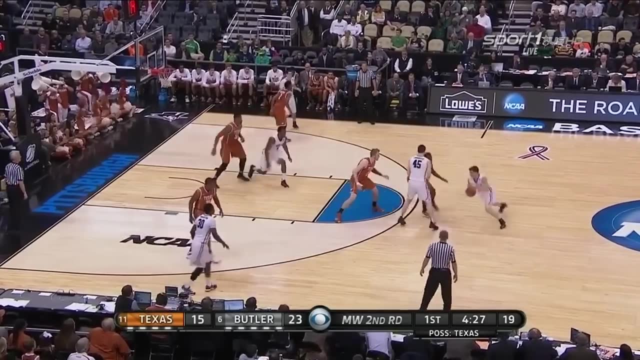 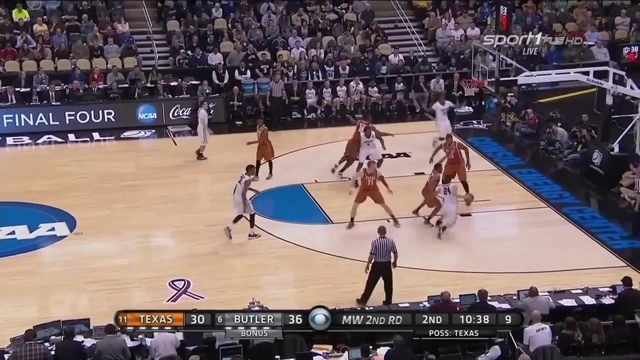 NCAA tournament with a victory over Wofford. to shoot outside jump shots: Dunham, that's a three go, got it. That is some kind of quick release in Kellen: Dunham Off. Dunham, little step back right, gets it in there. Martin gets the roll and a foul. 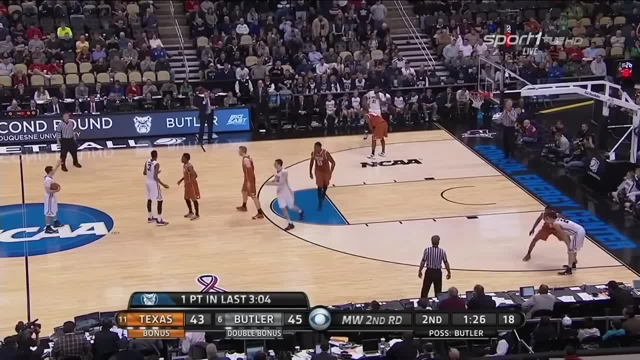 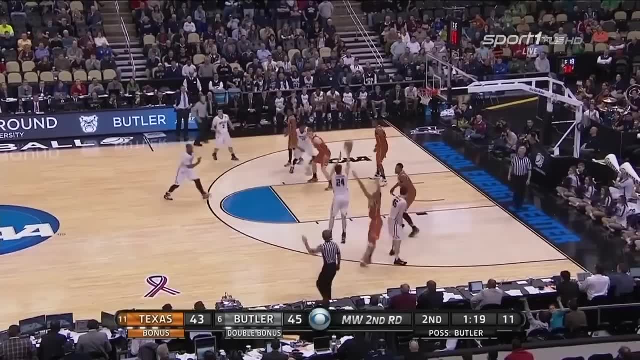 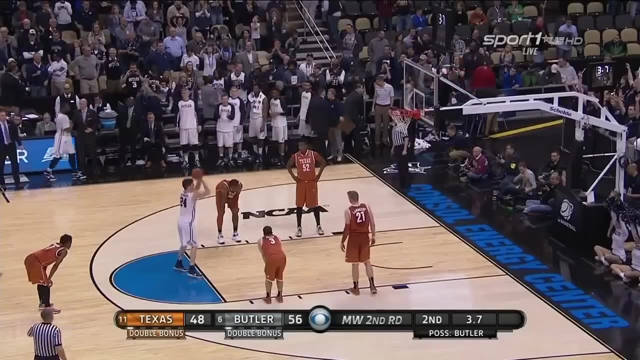 Kellen Martin flexing his muscles in the paint One point in the last three minutes and counting for the Bulldogs that one free throw by Dunham and Dunham buries a big one. So, Roosevelt-Jones, that's going to be a major story tonight and tomorrow as Butler gets. 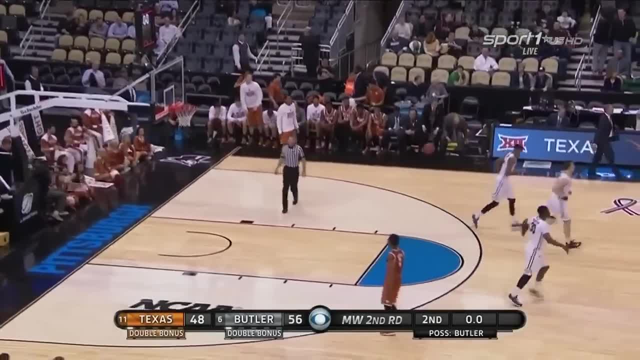 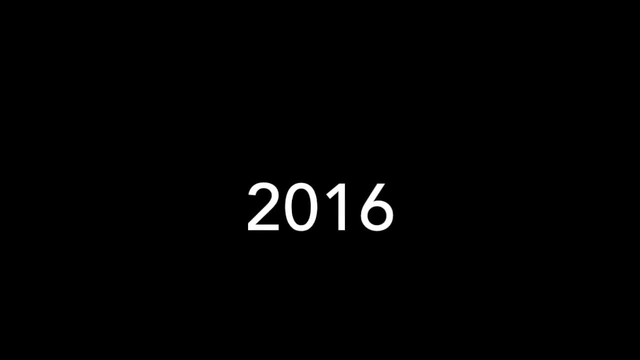 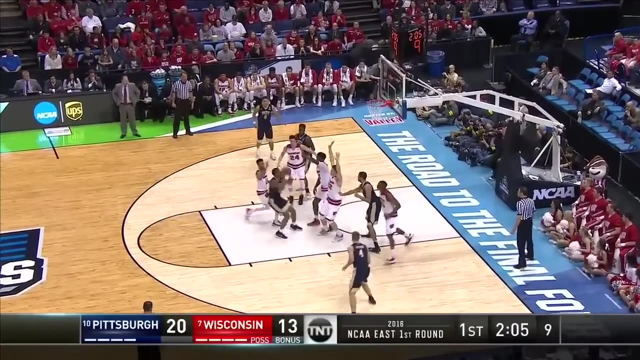 ready for Notre Dame. The Butler Bulldogs sending the Texas Longhorns home. the Big 12 is 0 for 3.. That went over Syracuse Curtis. back in there, Robinson, good ball. movement player: movement Jones, little tear drop. that was a pretty possession for the Panthers. 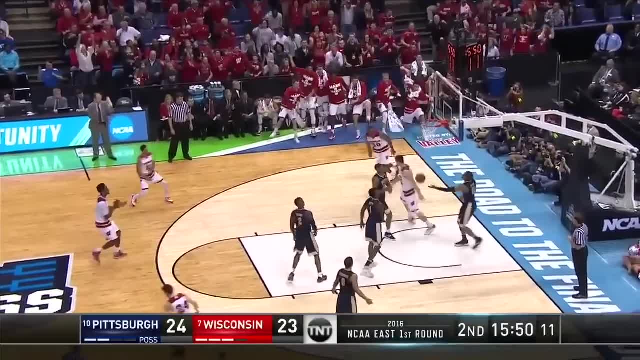 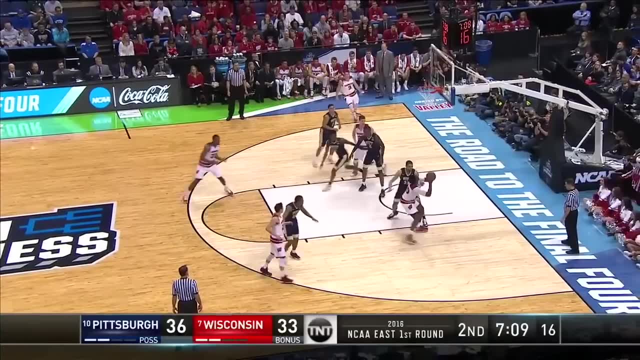 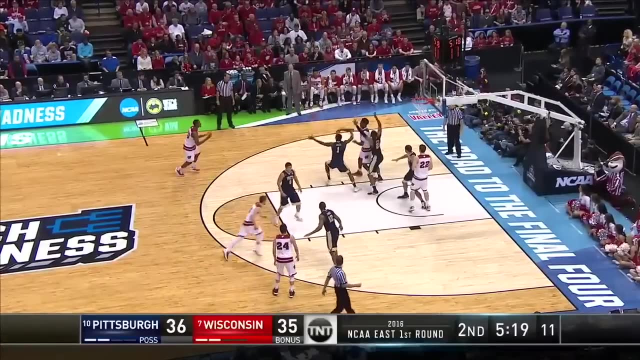 17-6 run since then and yes, 17-6 is a lot of points in this game: 25 points for the Badgers. Hayes patient and gets himself wide open with the left. Happa touchdown on block. Happa turns after a breather. Vito Brown hits a three. 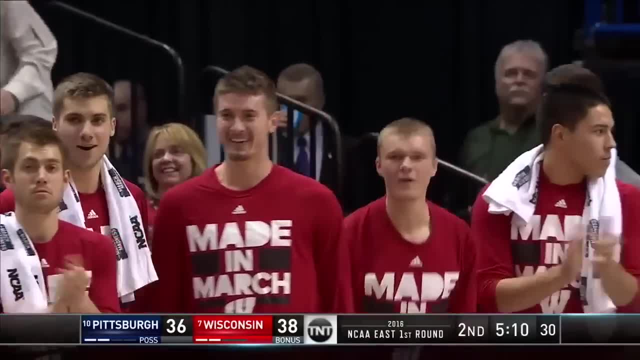 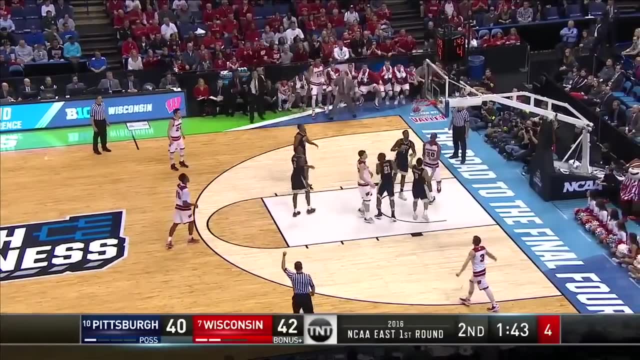 That's a big one for Wisconsin. they regain the lead. He's knocking down shots. Happa with the spin Geno was there for him this time, But if you don't double, he has some moves out there to make plays. 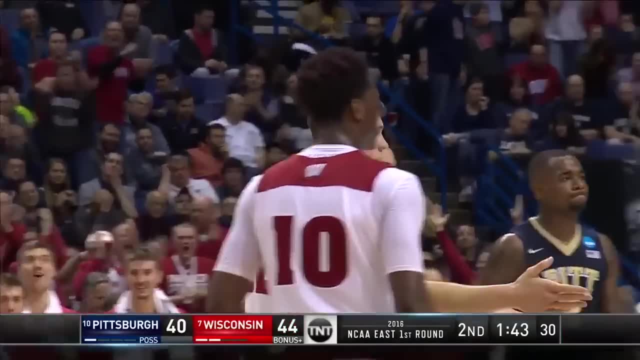 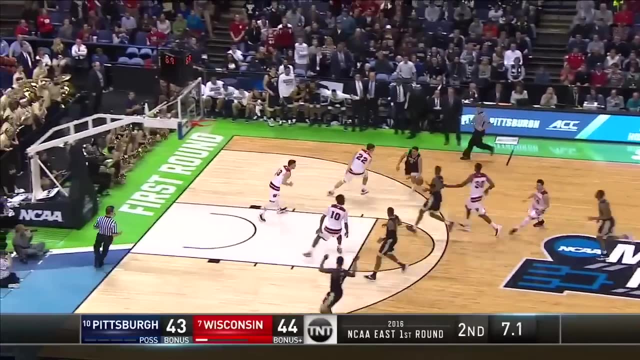 Oh it goes. and one for Ethan Happ: 90 yards shot. clock at three, Hayes rises up. oh, badly missed. and now Pitt with a chance. They're down a point. got a chance at the last shot, Robinson looking for a foul, he misses. 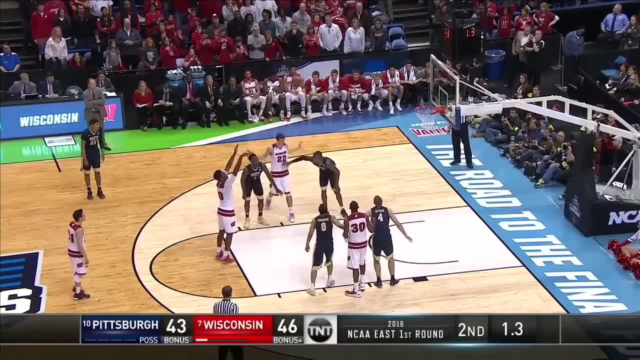 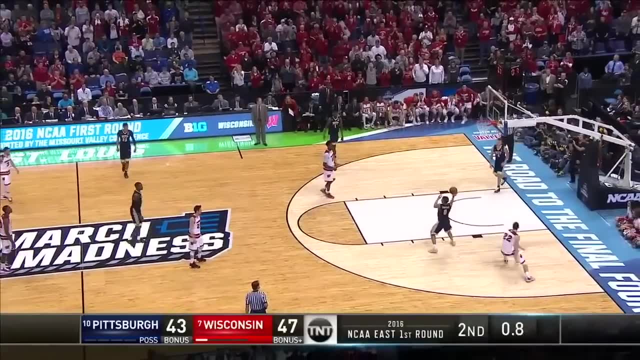 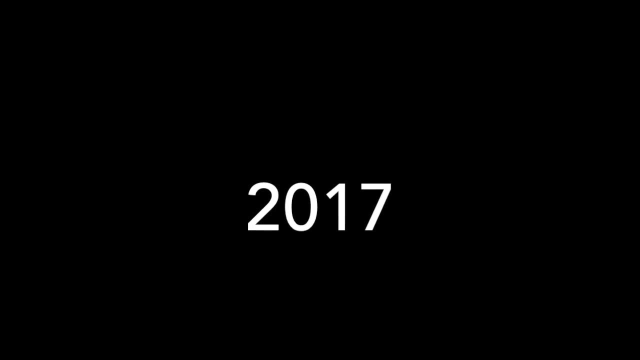 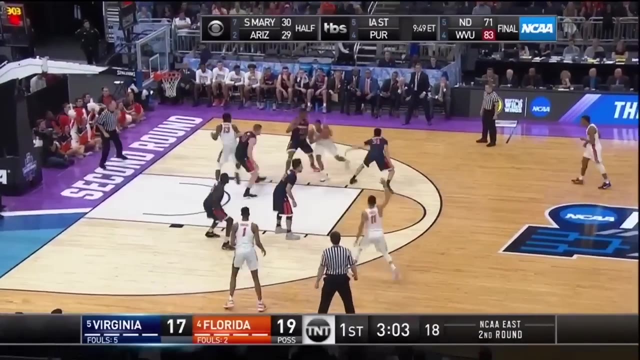 Ball's free. here's Happ and a foul 16-point first half of this tournament and a four-point lead for Wisconsin. The Badgers can let it roll and that is it. The Wisconsin Badgers survive a grinder. Ryan Jerome did not start. 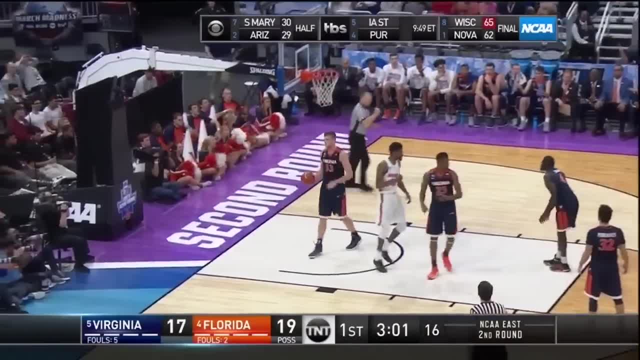 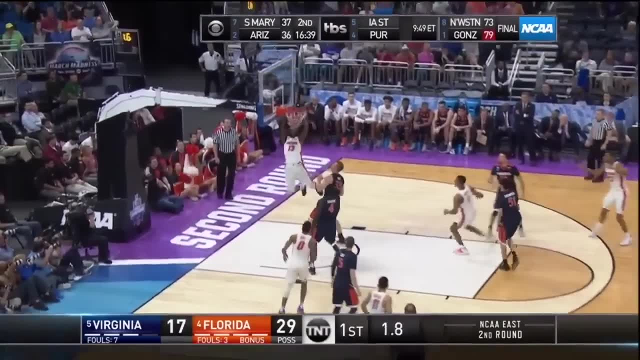 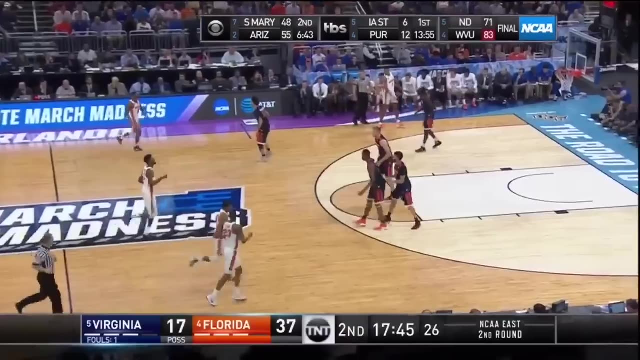 Leon, the drive, the flip, it's good. and a foul Switch. Hill with Shea Hill with three seconds, two seconds. Hill disses the slap. Calvarius Hayes beats the buzzer with a blast to the rim. 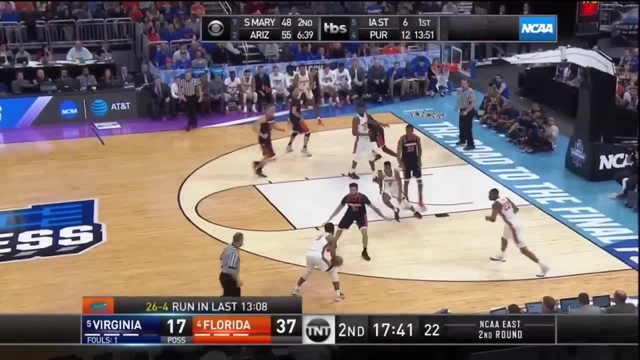 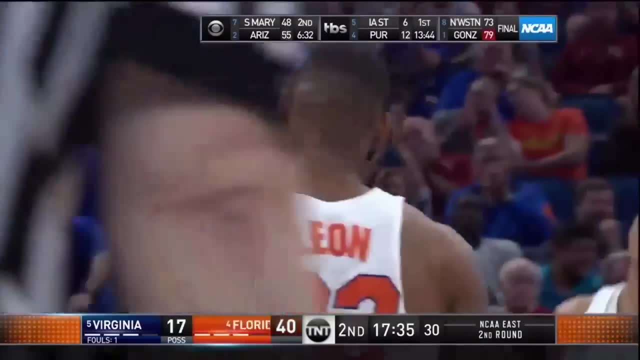 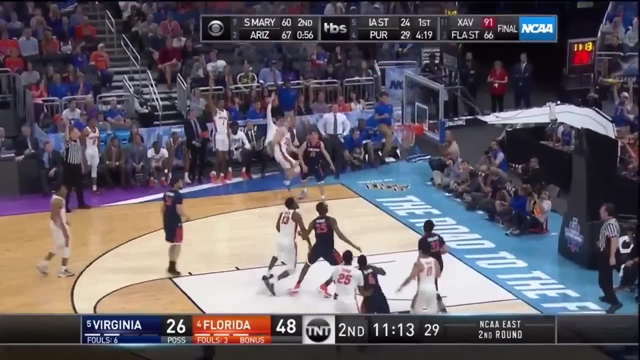 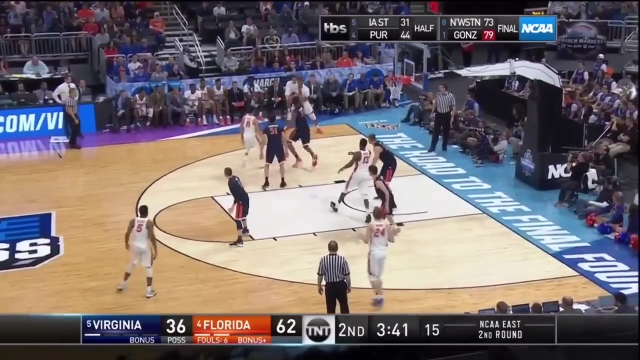 The not being tied together with the passing and catching The miss by Perrantes Leon. again, Justin Leon is lethal, But because of the size, the balance, the experience, Barry, a three Last game, 345, as the clock winds down, and all the elements. 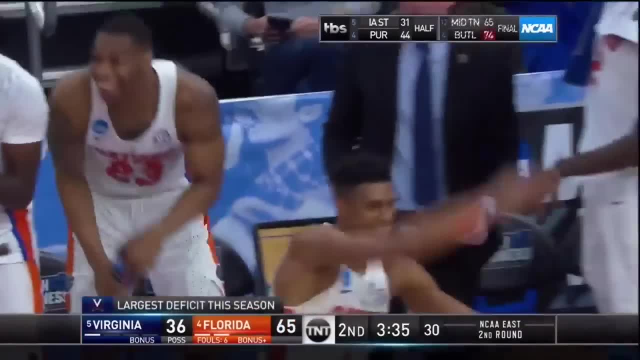 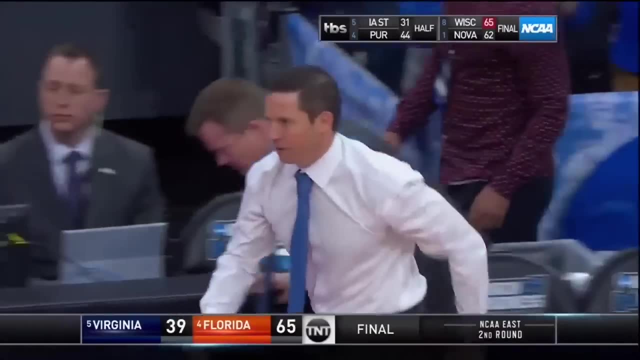 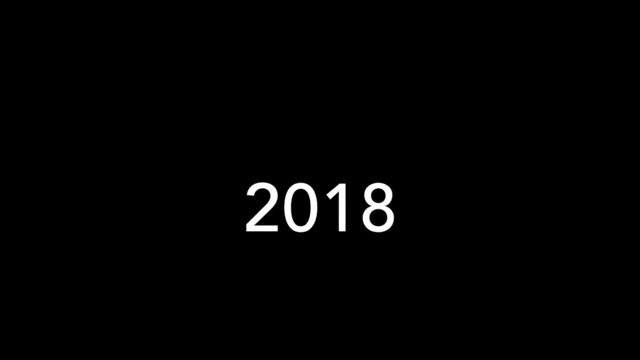 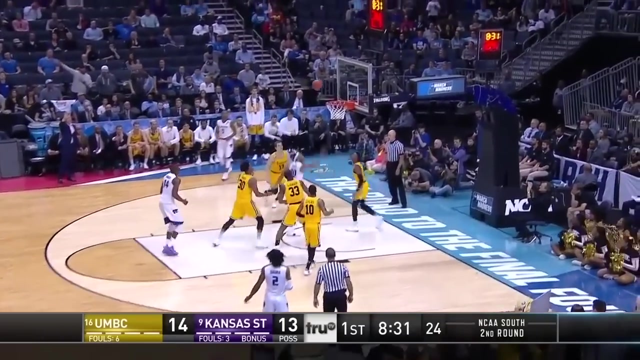 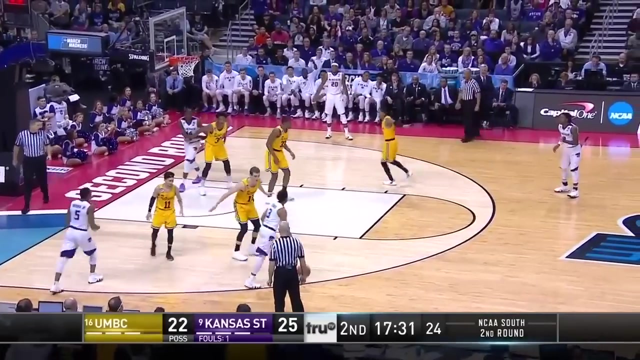 A three. Keith Stone Shot of the buzzer. Jerome Florida basketball. He is back. The Gators return to the Sweet Sixteen. Nice, slip with the hand there, got a piece Snead, drive it in and gets the bucket to go, and A-State has taken its first lead. 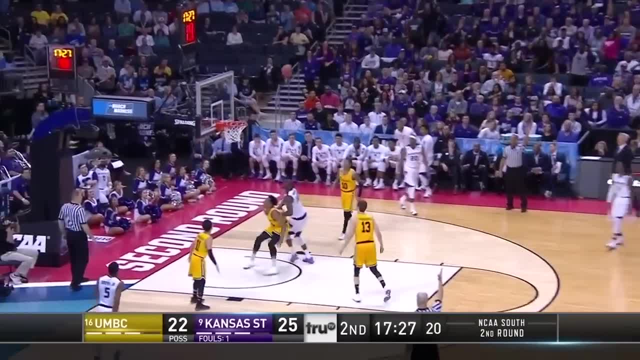 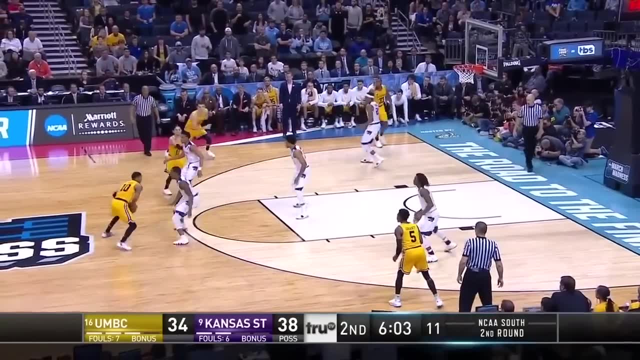 They have a lot of guys who can turn the corner and create nice step-back. Jada, how about this one? A little Southie drilling it? Kimora, back outside Miles, look at the field, He puts it up. 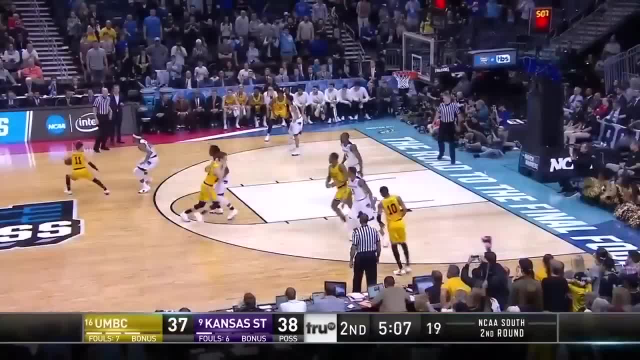 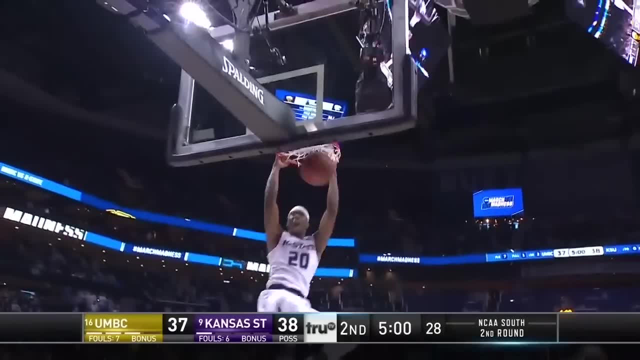 First shot of the second half, And it's a big one. With the penetration, Kimora has it stolen away, Snead. Kimora, get there in time. no Monster dunk Jumper, not the same, Oh, Snead. 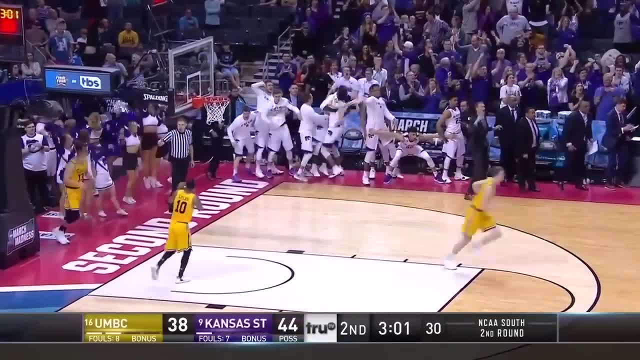 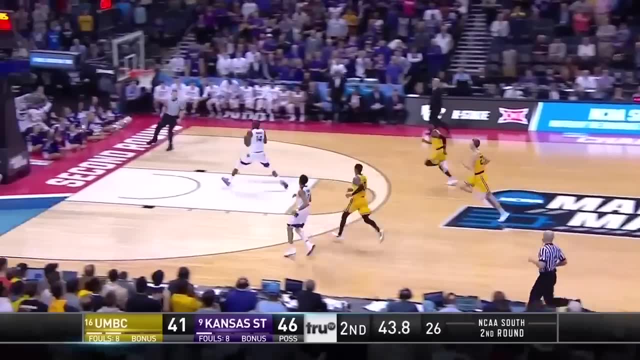 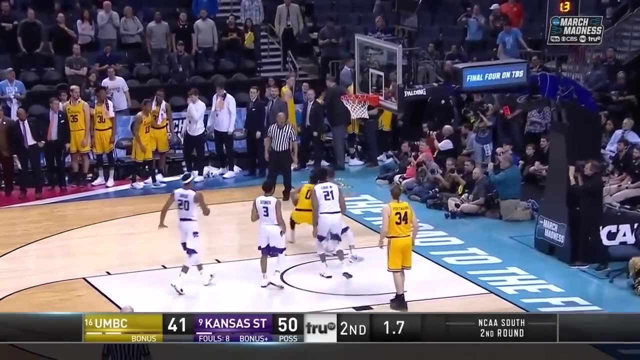 You saw it coming. That was nothing to Snead about. Back position. now Look up the other end. Look up the other end. They win, They get it to him and he dunks it down And it all comes to an end. but what a magical ride it was.